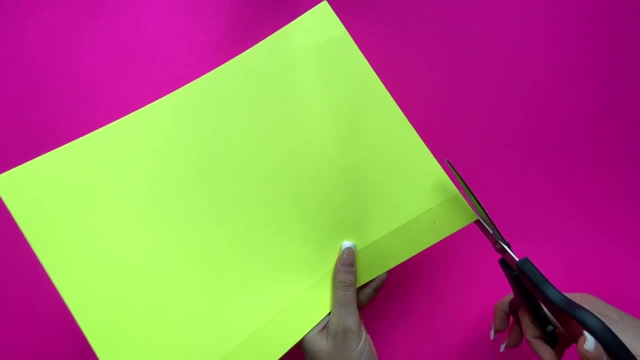 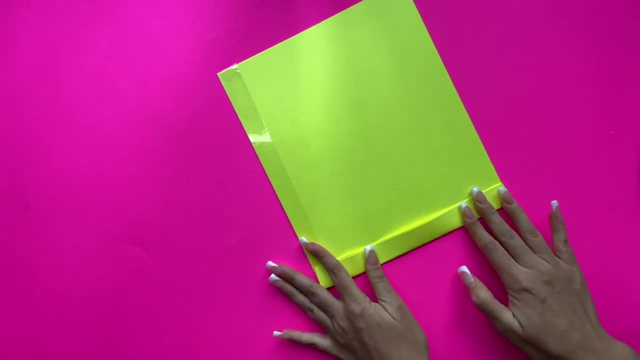 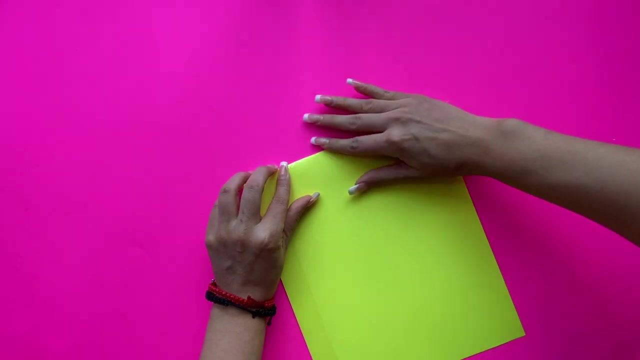 Now grab your scissors and cut any tape outside of the paper. Now go ahead and grab the top of your blind bag and make a fold about half an inch. After you fold it, go ahead and grab your tape and tape carefully Again. stretch out your tape pretty good, so there's no bubbles left. 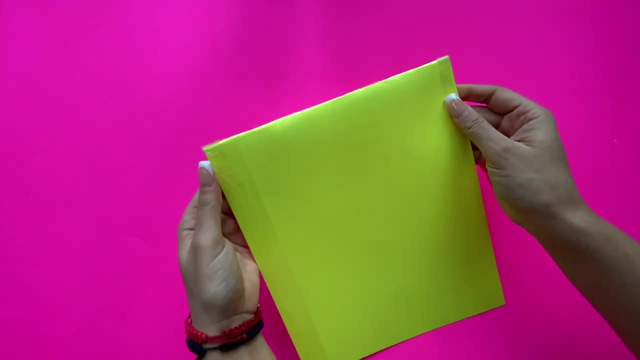 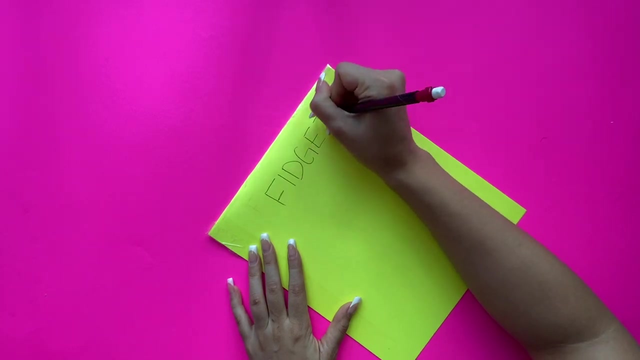 And for this tape that is left, I just fold it in. Now comes the fun part. sweeties, Time to get creative. Fun fact: this blind bag can be used for many things, not necessarily fidgets, but in this channel. 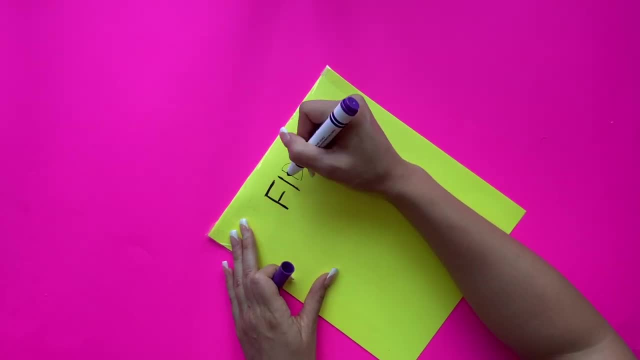 we love fidgets, so we had to do it. As I am adding fidget toys, I realized the letters were a little small, so I went ahead and erased. I recommend using a paper towel to remove the tape. I recommend using a paper towel to remove the tape. 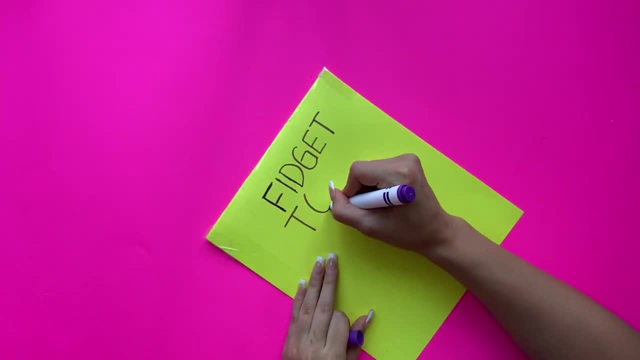 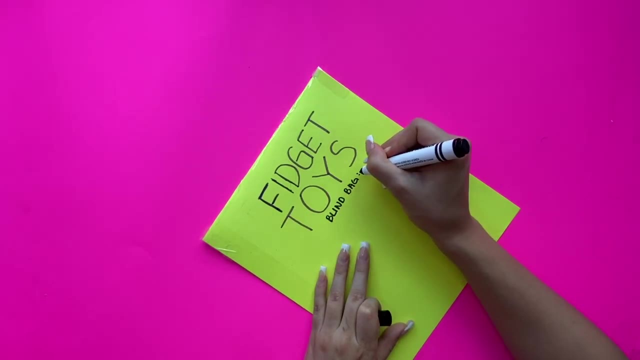 I recommend using a paper towel to remove the tape. I recommend using a letter pencil to trace. in case you messed up like I did Now below fidget toys, I will write down blind bag And with my markers I'll go ahead and make some designs to make this blind bag look extra cute. 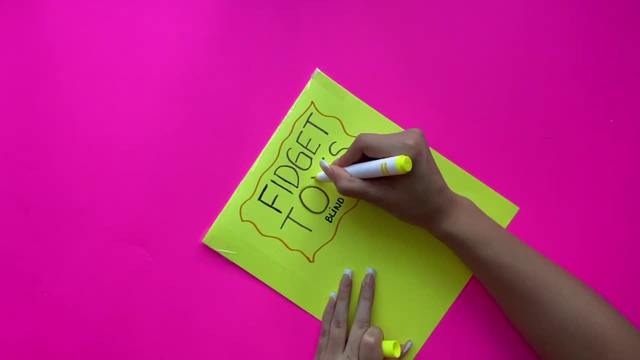 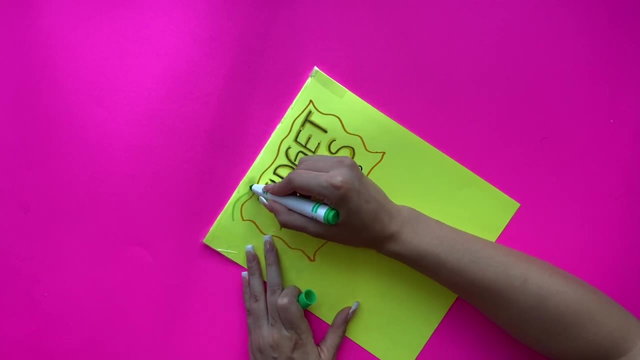 I grab my yellow marker and will trace one more time the letters so it can pop even more. Something I really like- sweeties about these blind bags- is that you can get as creative as you like. You can make this a summer blind bag. 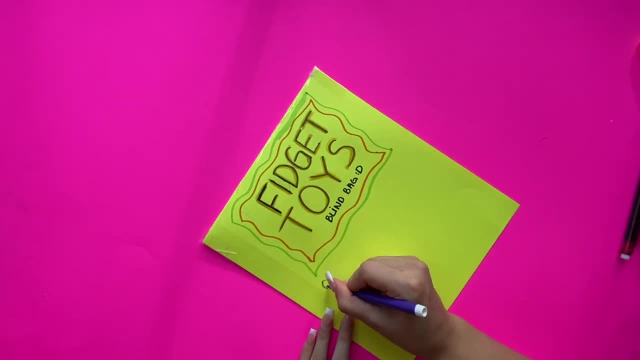 blind bag, a winter blind bag or anything you like. I will add four type of fidgets that I could get. I could get a common fidget, an uncommon fidget, I could get an ultra rare fidget or a. 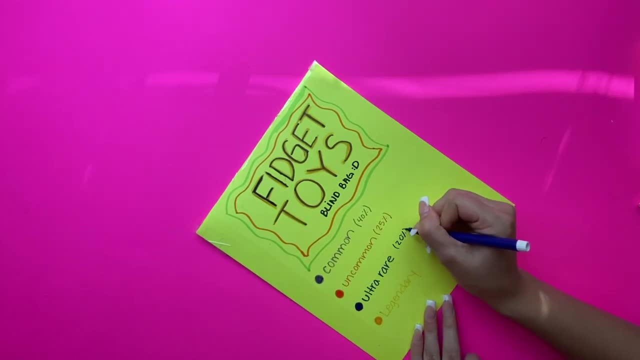 legendary fidget. To make it more fun and interesting, I will add a percentage to each one. As you can see, it is more likely to get a common fidget than a legendary fidget, but we will see. I will be having three fidgets inside of this blind bag and if I turn to the back, 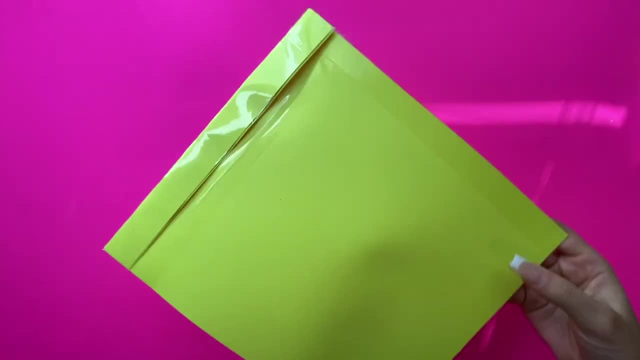 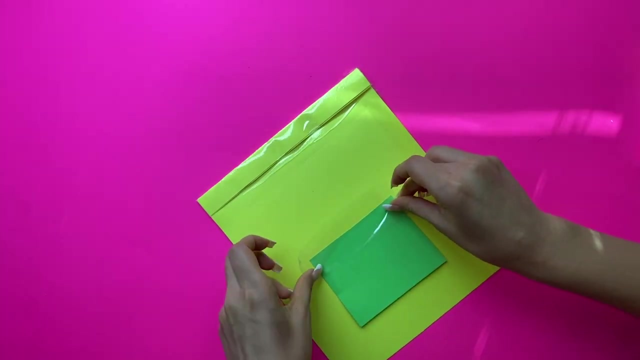 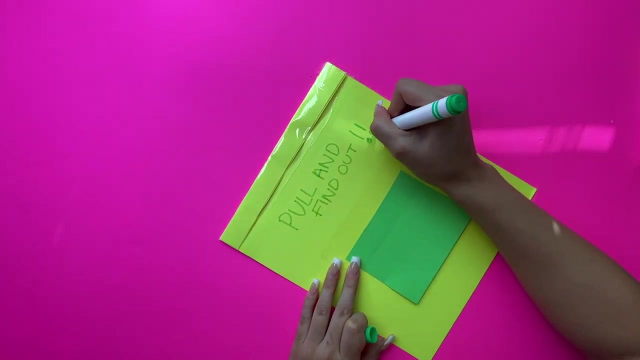 I will find. what type of fidgets will I'll be getting? Let's turn to the back and go ahead and grab another paper and cut a square, not too big, not too small. Go ahead and place it at the bottom and tape it. Now let's go ahead and write the instructions, which is pull and find out. I'm 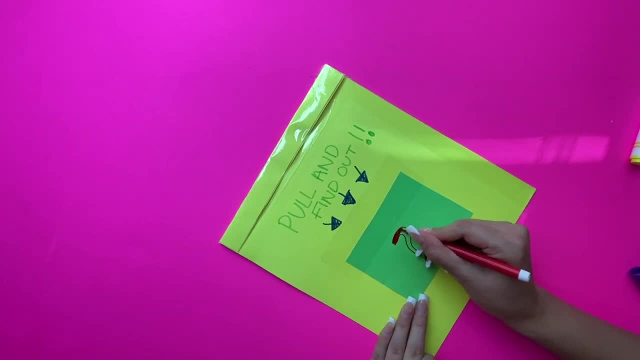 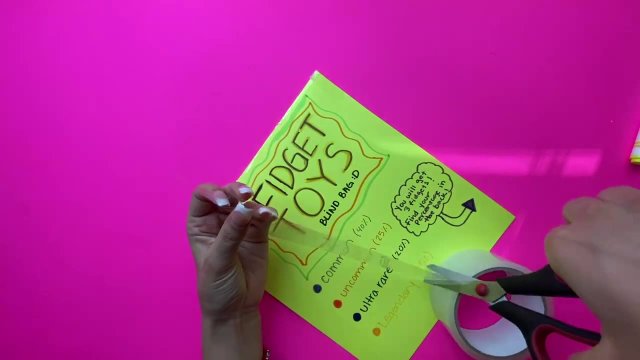 adding some errors as long as they question mark. I've decided that for this blind bag, we'll be having ultra rare fidgets. So now that this is done, sweeties, it's time to open the blind bag. I'm going to open the blind bag and I'm going to open the.